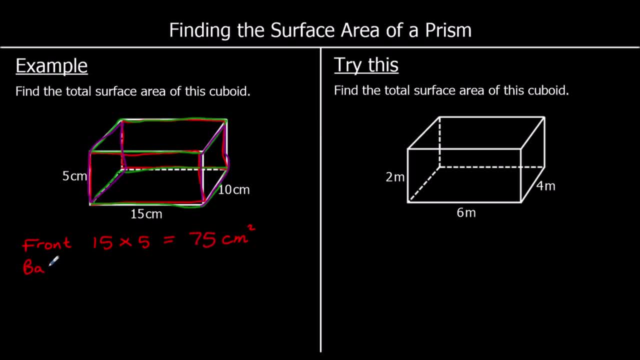 The back is identical, so the area of the back is also 75 centimetres squared. For the top again, we've got a rectangle, the top or the bottom, which is 15 by 10.. So 15 times 10, which is 150 centimetres squared. 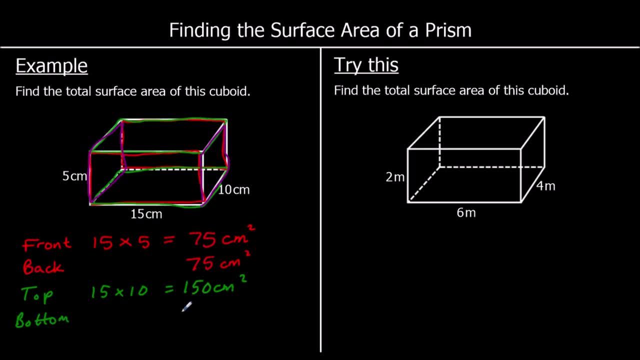 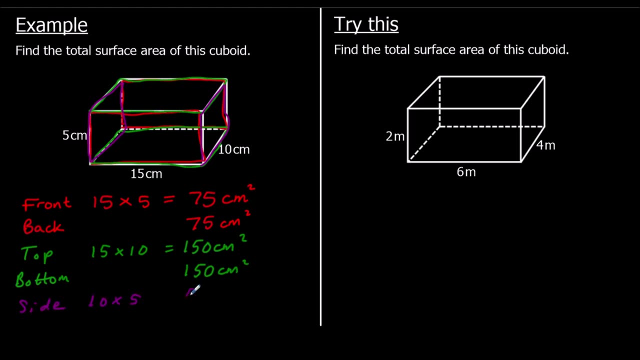 The bottom is identical to the top And the side, so it's 10 by 5, which is 50 centimetres squared, and again there are two identical sides, So they both have an area of 50 centimetres squared. 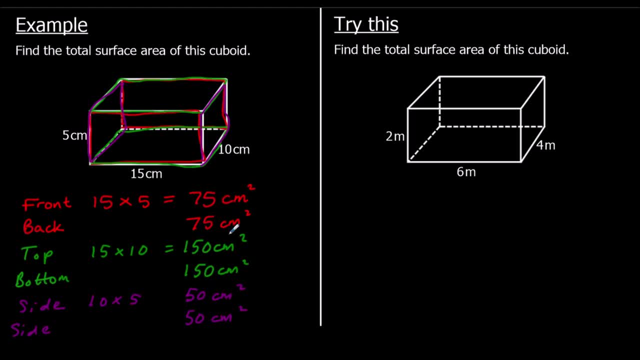 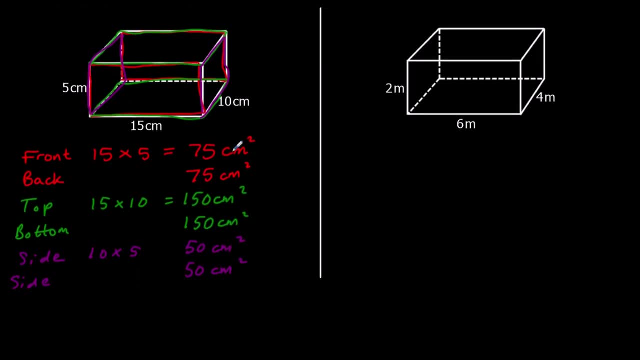 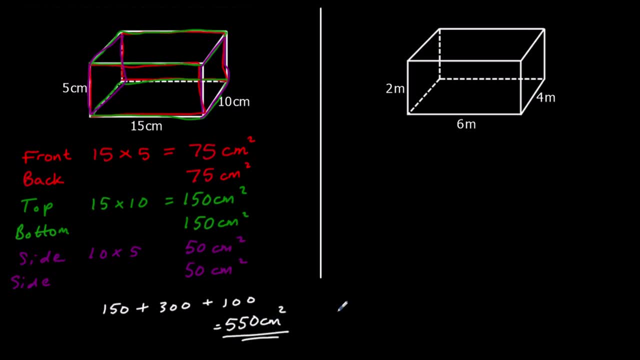 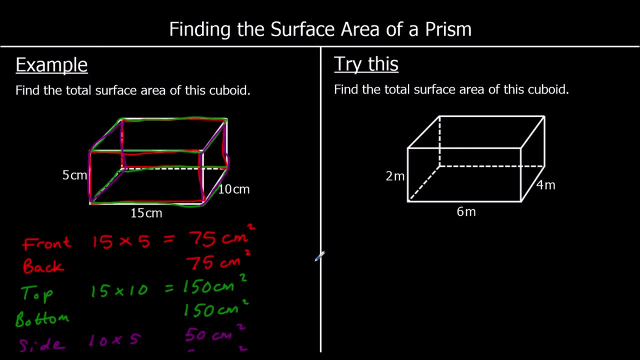 squared, so the total surface area is 550 centimeters squared. okay, one for you to try. so find the total surface area of this cuboid. so there are going to be six surfaces again. so let's start with the front. and that is six times two, which is 12 meters squared. 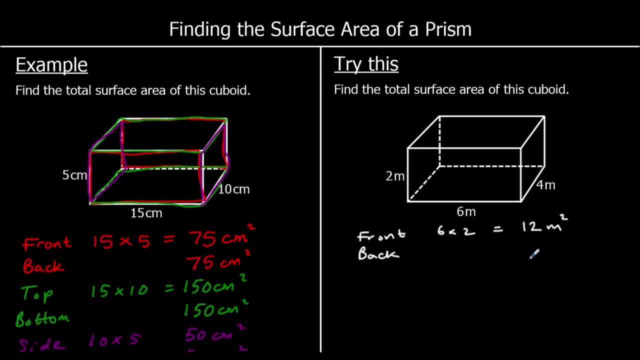 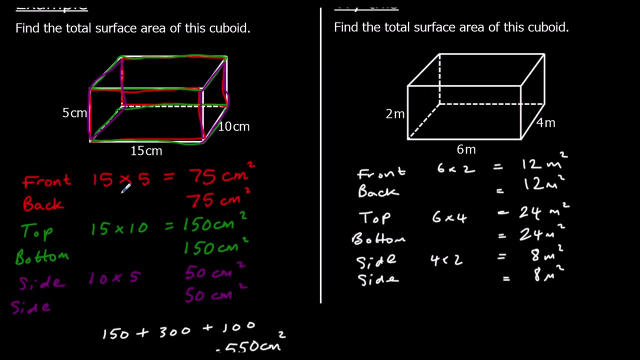 the back is exactly the same as the front, so it's also 12 meters squared. the top and the bottom are 6 times 4, which is 24 meters squared, and the side is 4 times 2, which is 8 meters squared. meters squared, and the other side is also 8 meters squared. so we need to add 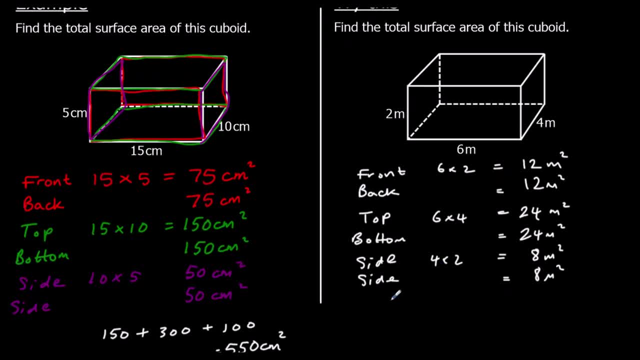 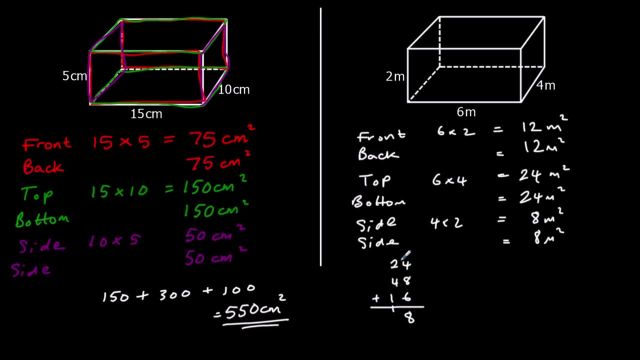 these together. so 2 x 12 is 24,, 2 x 24 is 48,, 2 x 8 is 16, and we'll add them up. so 4 plus 6 plus 8 is 18, 2 plus 4 plus 1 plus 1 is 8, so we've got 88 meters squared. 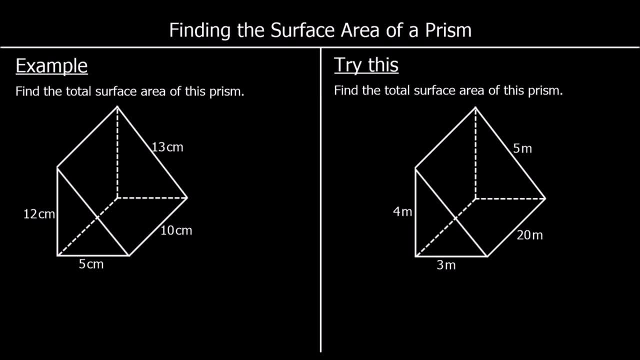 here's a different question. this time we've got a different shape, but we're still going to find the area of every surface and add them all together. we've got 8 x 12 is 18, and we've got 4 x 6 is 18, and we've got 6 x 12 is 18 and we've got. 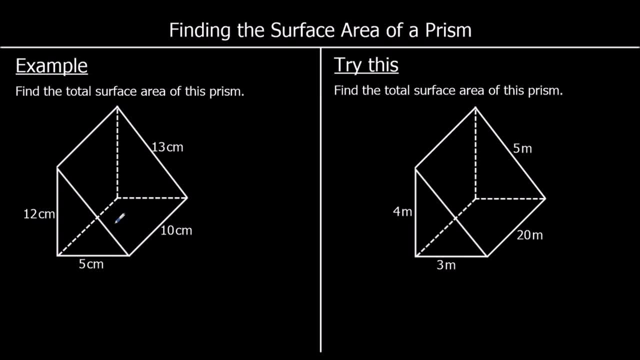 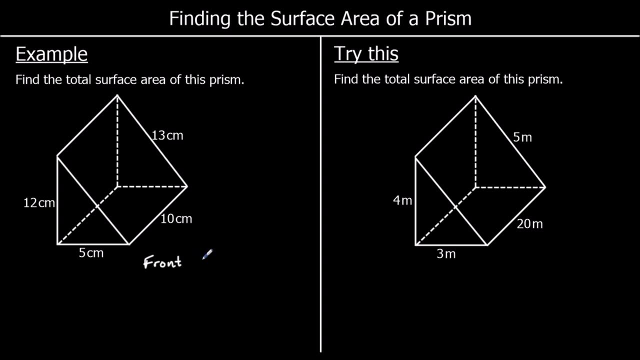 got a triangle. on the front and the back They're identical triangles. So we've got two of those triangles, but then we've got three completely different rectangles that we need to add together. So the front, the area of a triangle, is the base times height. 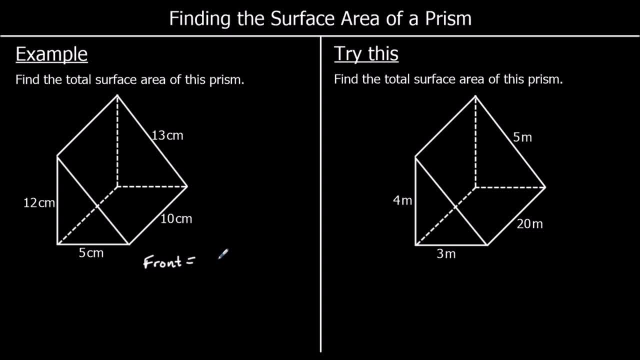 divided by two or half base times height, So it's half of five times 12, which is the same as five times six, which is 30 centimetres squared, And the back is also going to be 30 centimetres squared. They're two identical triangles on the front and the back, The bottom. 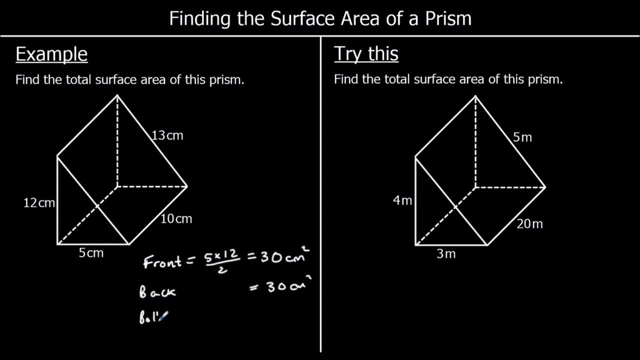 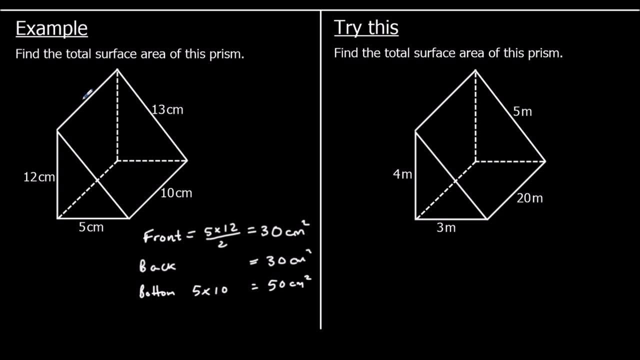 is five times 10.. So five times 10,, which is 50 centimetres squared. We've got a triangle on the front and the back We've got a slanted side. So a slanted side is 10 times 13,, so 130 centimetres squared. 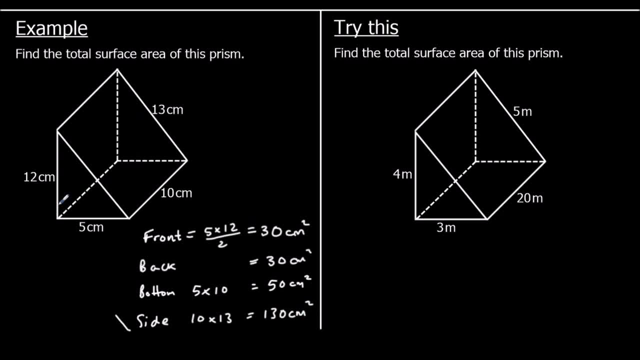 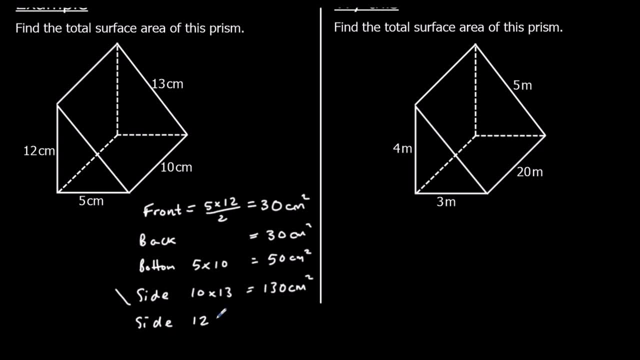 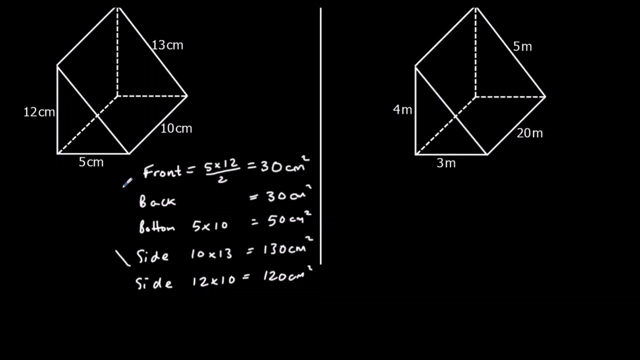 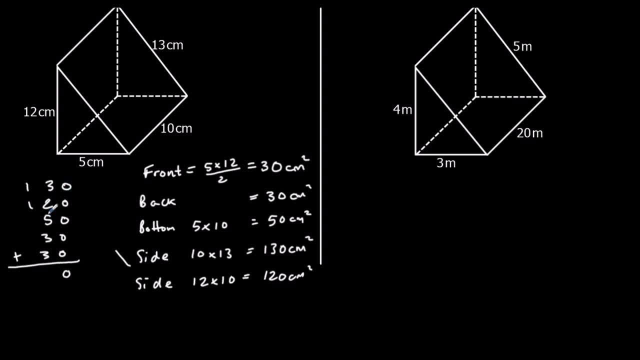 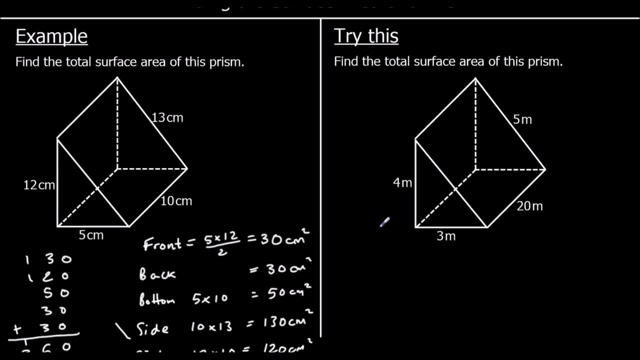 Okay, one for you to try, So give it a go. Okay, So we've got identical triangles, two identical triangles. So we've got the front and the back, which are going to be half base times height, So half times four times three, which is six metres squared this time. So the front and the back. 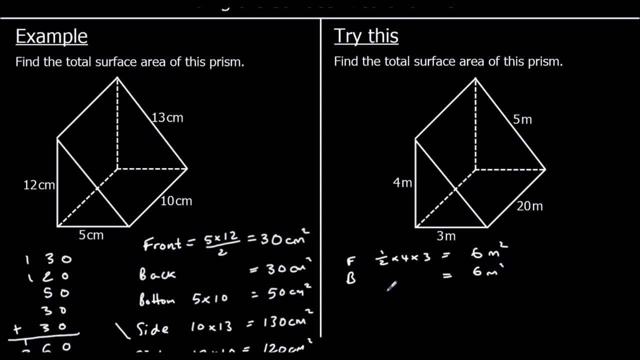 are six metres squared. Our the bottom is three times 20,, which is 60 metres squared. The slanted side is 20 times five, which is 100 metres squared, And the straight side is four times 20,, which is 80 metres squared. So what do we have in total? We have so 180 plus 60 is 240,. 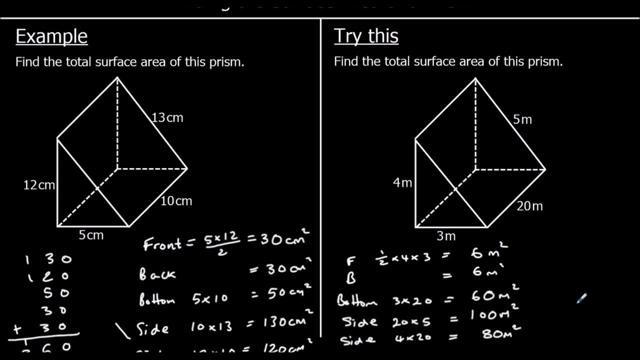 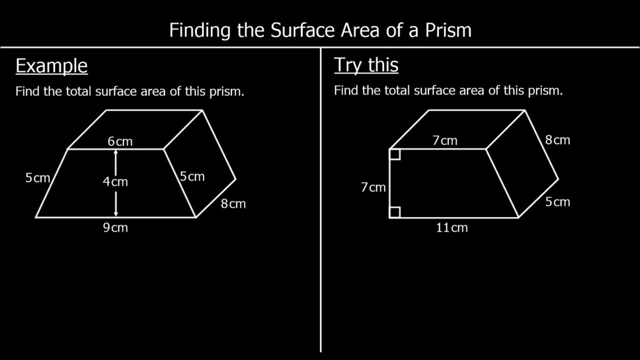 plus 60,, which is 180, plus 60,, which is 240.. So we've got a total of 40 metres squared. So we've got 12, so 252 meters squared. okay, another surface area question. so it's still adding up the area of every surface. this time we've got a trapezium on the front. 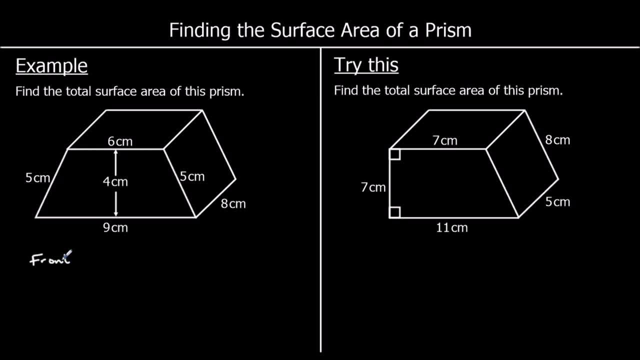 so we've got an identical front and back. so the front is the area of the trapezium which is half the sum of the parallel sides times the distance between them. so 6 plus 9 is 15, half of 15 is 7 and a half, and then 7 and a half. 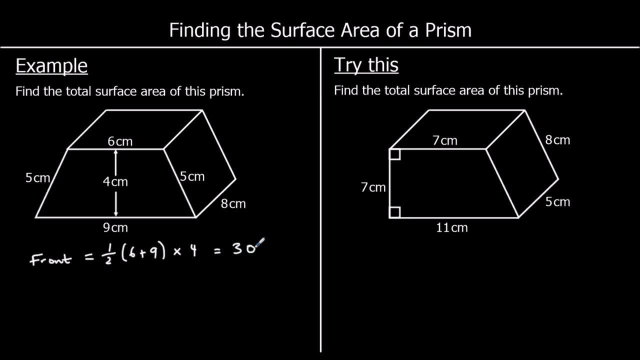 times 4 is 30, so we've got 30 centimeters squared. the back is identical, so the back is also 30 centimeters squared. the two sides are identical. they're both 5 times 8, which is 40 centimeters squared, so both sides of an area of 40 centimeters squared. and 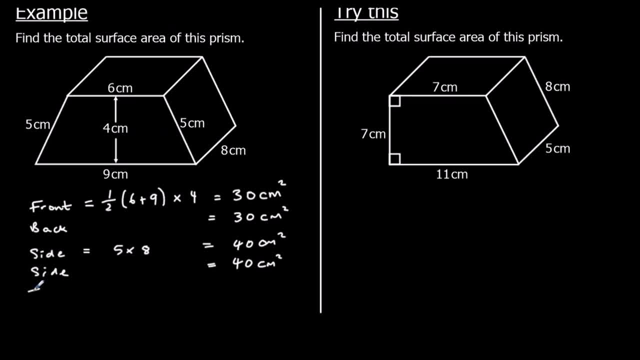 the top and the bottom have got different areas. so the top is 40 forsame 32 centimeters squared, which is 0.oli negative cal weapon times 4, which means it Internet each side times 1 of 8 C, So this becomes 14 plus 8. 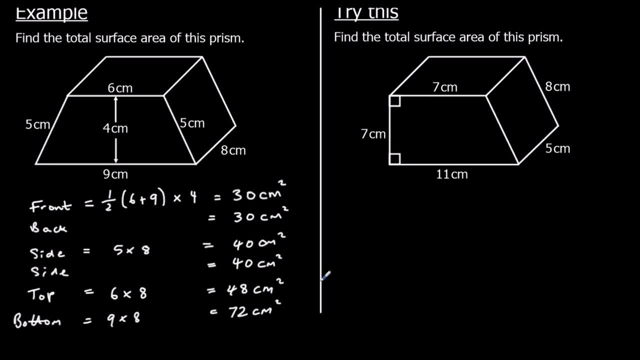 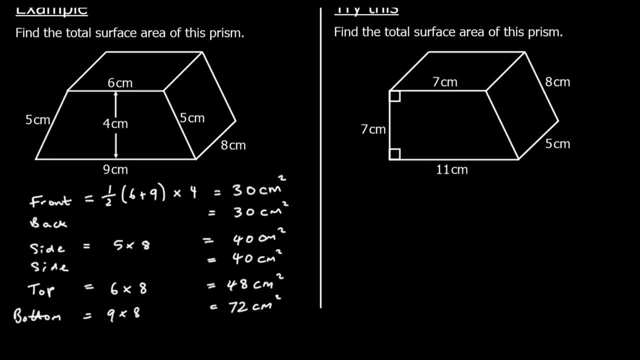 six-eighths, which is 48 centimeters squared, and the bottom is nine-eighths, which is 72 centimeters squared. so we've got one, two, three, four, five, six surfaces: six-eighths, which is 48 centimeters squared, and the bottom is nine-eighths. 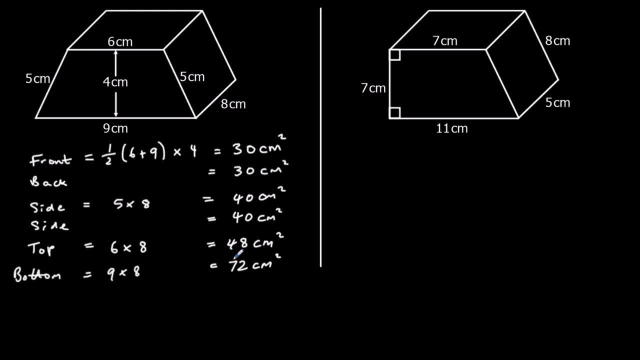 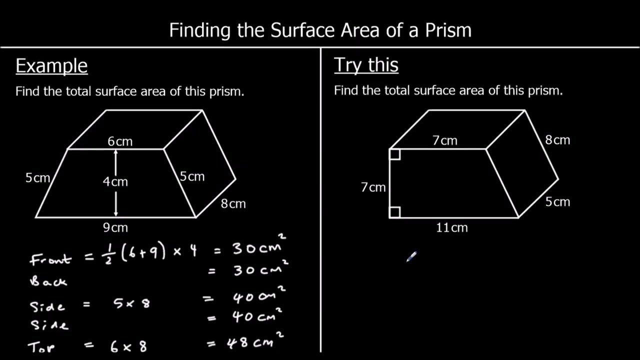 2 plus 48 is 120, plus 80 is 200, plus 60, 260.. So we've got 260 centimetres squared And one for you to try here, so give this one a go. Okay, this one's slightly different to the last one, but we've still got a trapezium on the front. 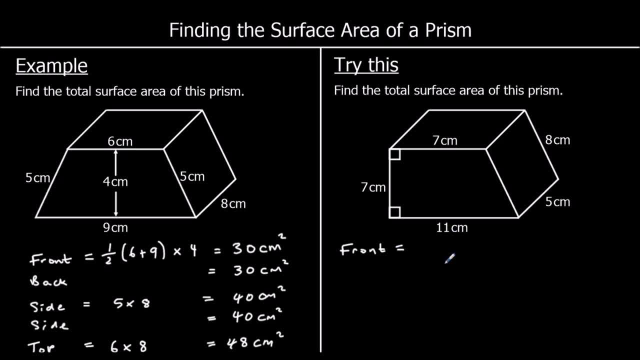 So the front is going to be half the sum of the parallel sides, so half of 7 plus 11, times the distance between them, which is 7.. 7 plus 11 is 18, half of that is 9,, so 9 sevens are 63.. 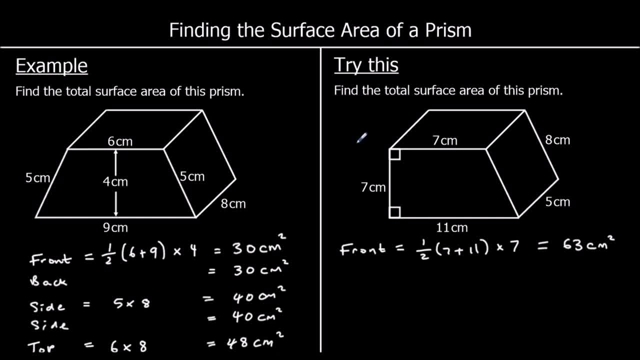 So 63 centimetres squared is the area of the front shape. The back shape is exactly the same. Now the other sides are all going to be different. Well, so the top is 7 times 5, which is 35 centimetres squared. 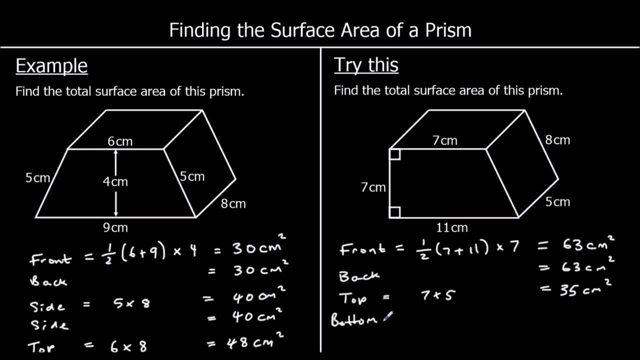 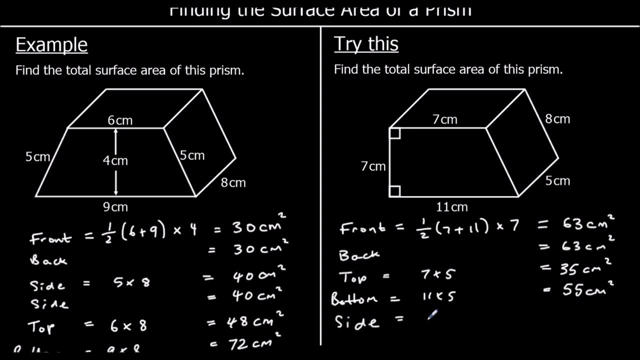 The bottom is 11 times 5,, which is 55 centimetres squared. We've got two sides that are different, So the slanted side is 8 times 5,, which is 40 centimetres squared, And the straight side is 7 times 5,, which is 35 centimetres. 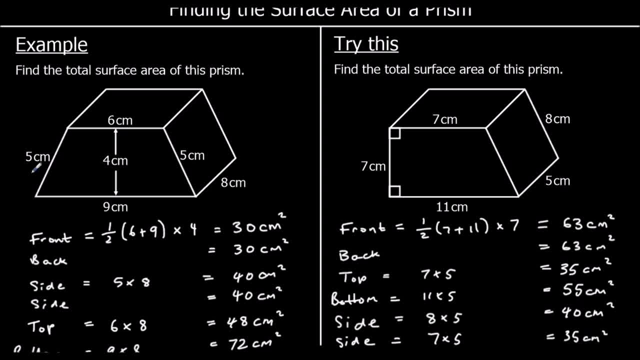 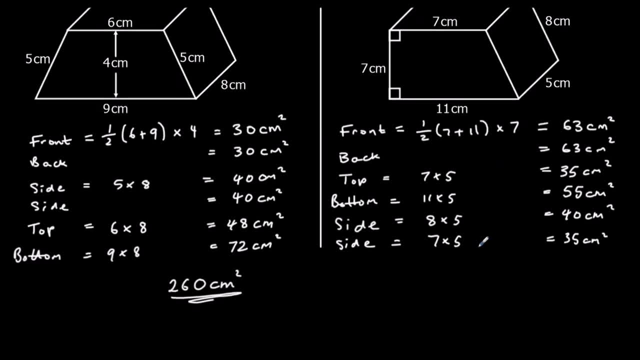 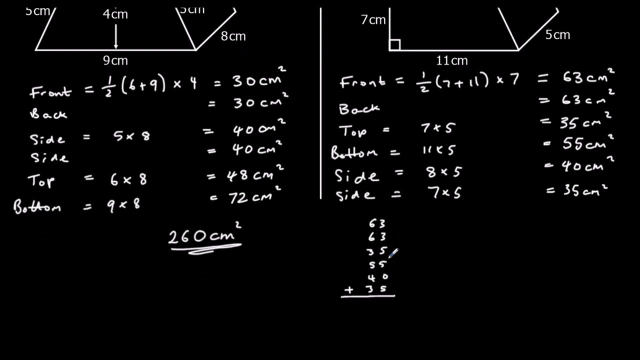 So we want the total surface area. so all of these areas, the area of every side added together, And I'm just going to write them down and add them up in the columns. So we have 5 plus 5. plus 5 is 15, plus 3 is 18, plus 3 is 21.. 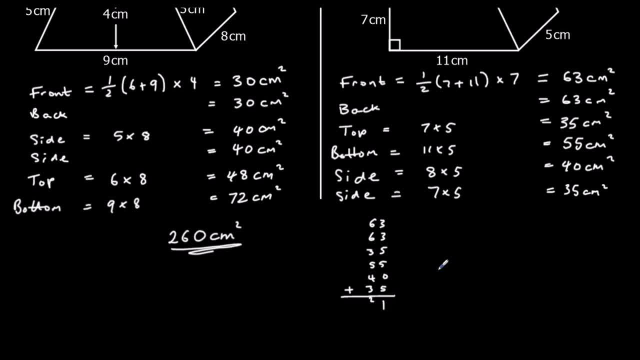 So 1 and the 1s carry over the 2. And we've got 6 plus 6,, which is 12, plus 3,, which is 15, plus 5,, which is 20, plus 4, plus 3, plus 2,, so 29.. 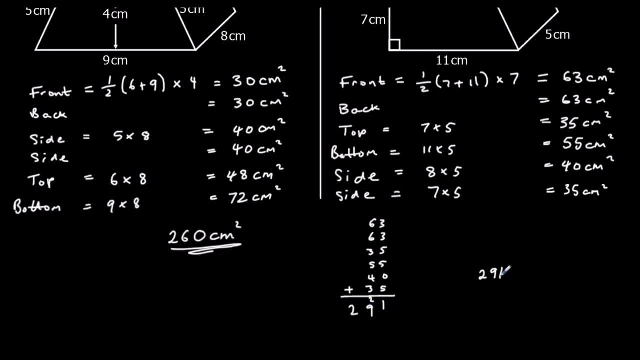 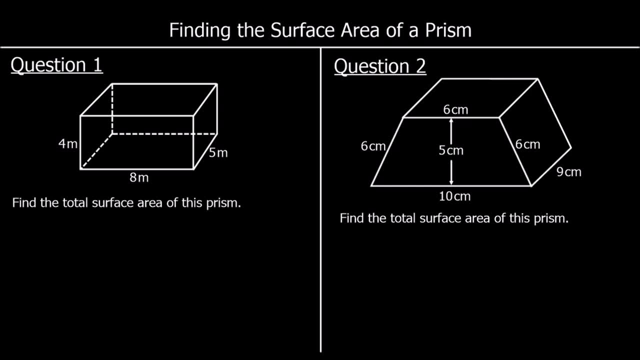 So we've got 291 centimetres. And to finish up, we've got two questions. So pause the video, give them a go. So question one: find the total surface area. So we've got the front and the back, which are identical. 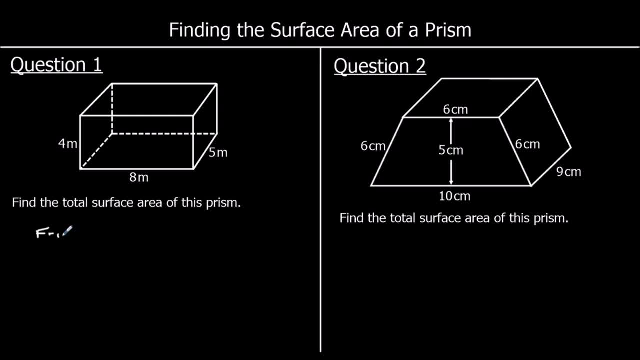 Which are both going to be 8 times 4.. So that's 32 metres squared. The back is the same. The top and the bottom are identical. They're both 8 times 5.. So that's 40 metres squared. 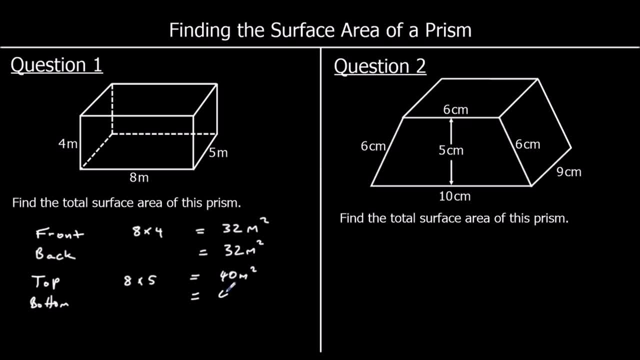 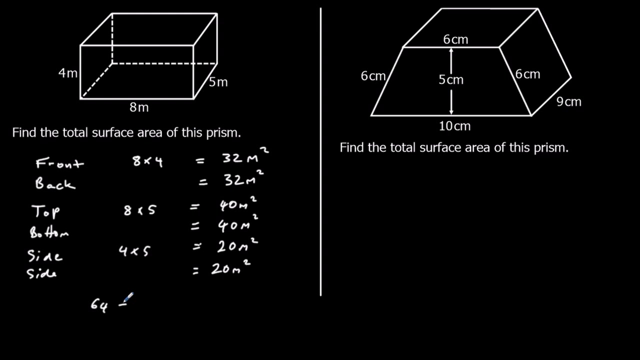 So the top and the bottom are both 40 metres squared And the sides are both going to be 4 times 5. Which is 20 metres squared. So if we add all these together, we've got 64, plus 80, plus 40..